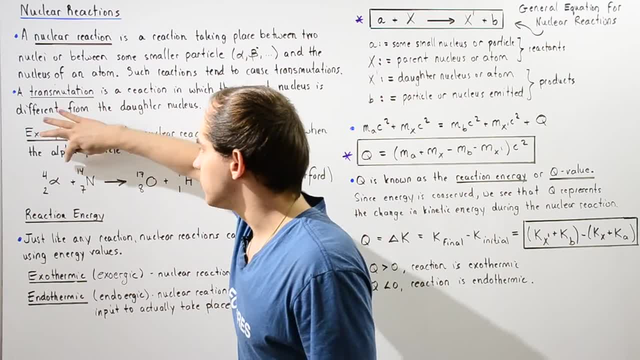 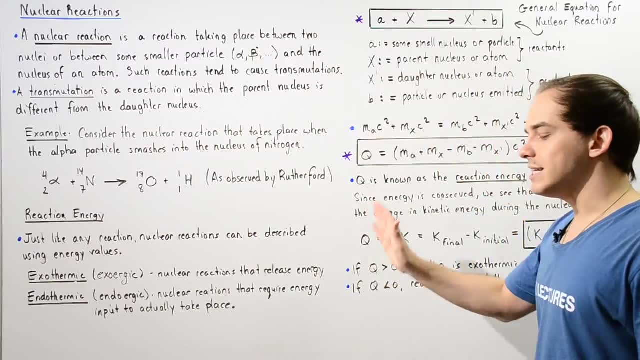 reactant side. The nucleon number is 4 plus 14 or 18 on the reactant side and the nucleon number is 17 plus 1 or 18 on the product side. So we see that the law of conservation of nucleon number 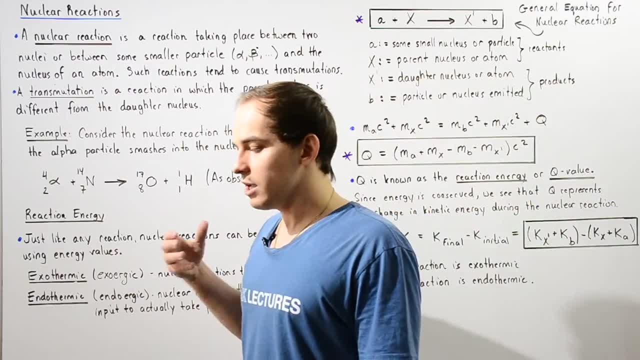 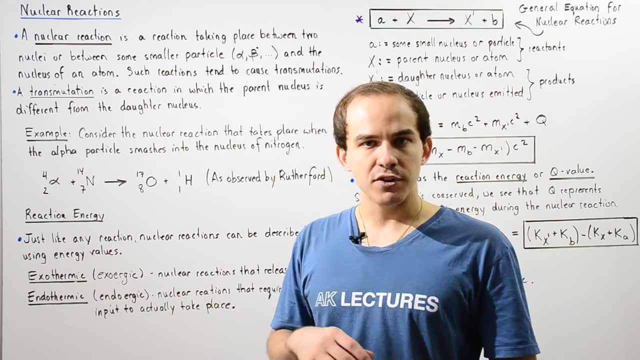 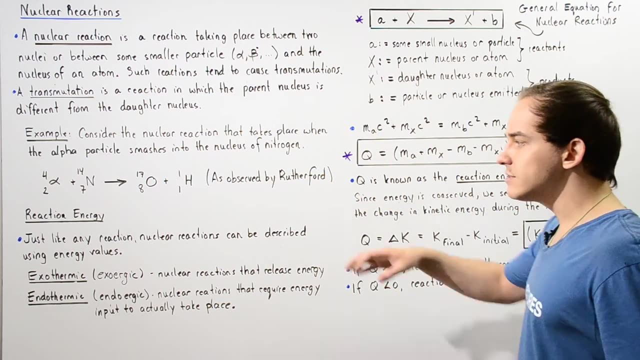 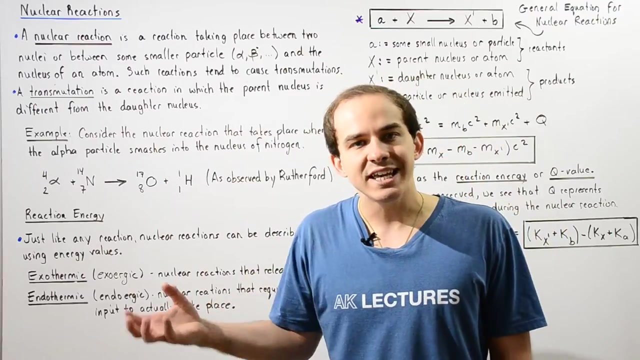 does in fact hold in our nuclear reaction. Just like we can describe the change in energies of the reactants and the products in any reaction, we can also describe the change in energy take place inside nuclear reactions. Now, if inside our nuclear reaction energy is released as a result, such a reaction is known as an 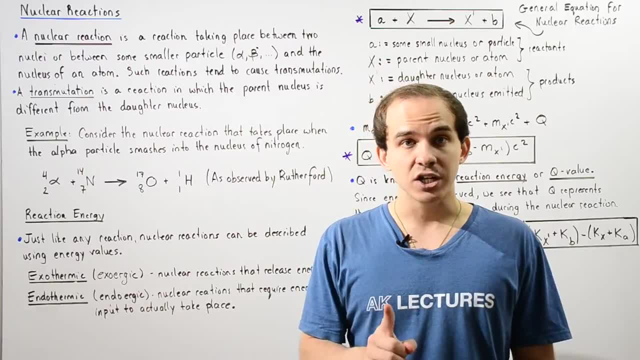 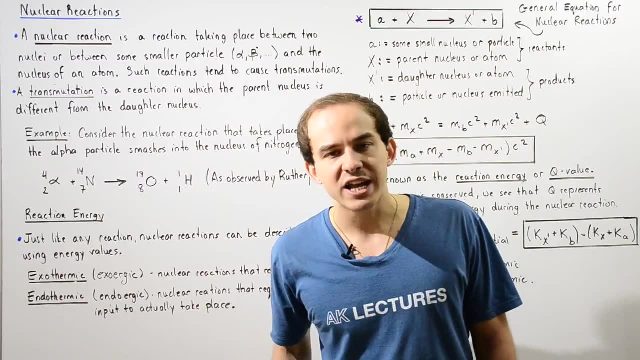 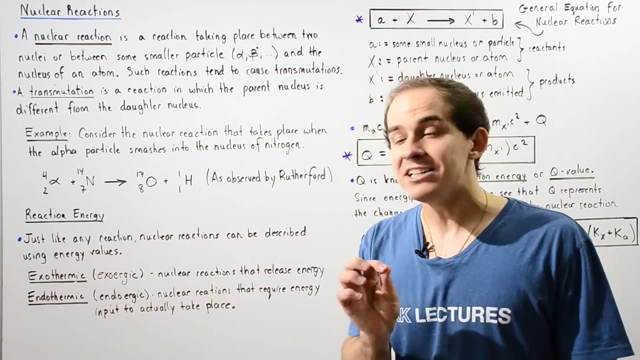 exothermic or an exoergic reaction. However, if in our nuclear reaction an energy input is required for that reaction to actually take place, such a nuclear reaction is called the endothermic or endoergic reaction. So basically the formula or the equation that 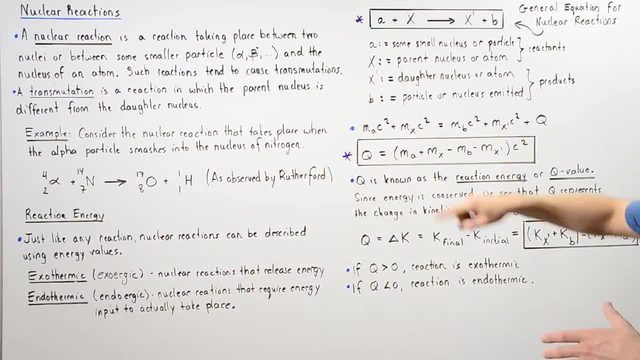 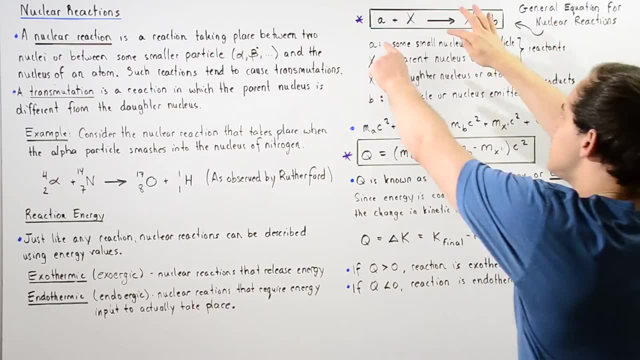 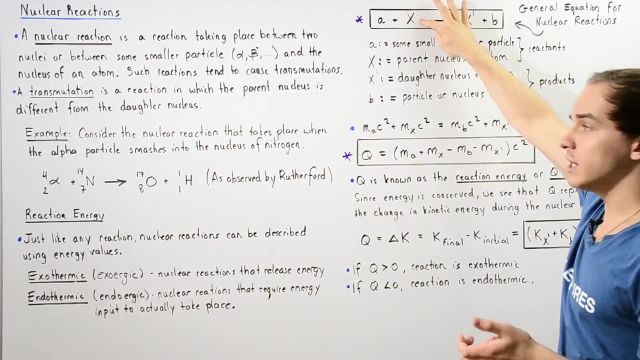 describes any type of nuclear reaction is given by this equation here. So this is the general equation for nuclear reactions. So we have the reactants collide to form the products. On the reactant side we have the parent nucleus or atom given by X, and our small nuclei or 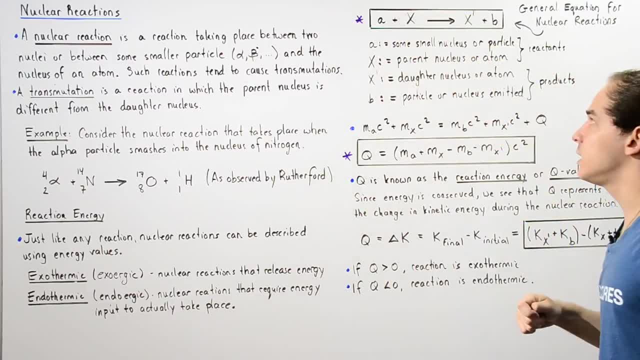 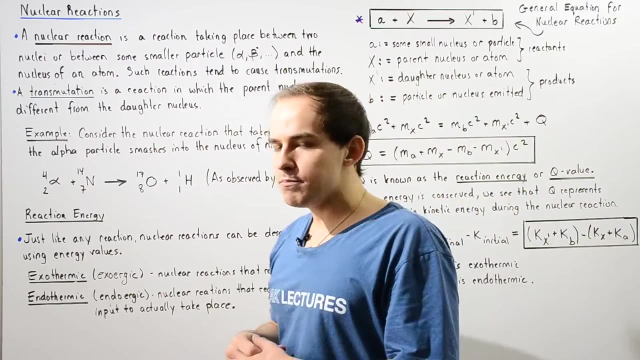 particle that collides with that parent nucleus. Now, on the product side, we have the daughter nucleus that is formed, given by X prime, and our small nucleus or particle that is released as a result. Now, as mentioned before, we have the law of conservation of energy that readily 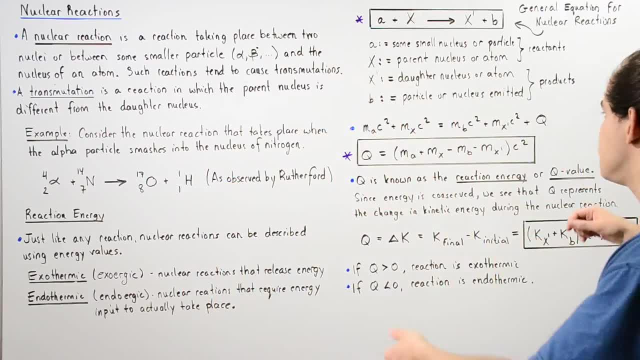 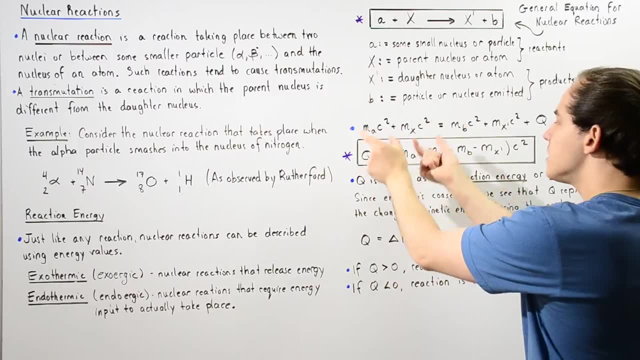 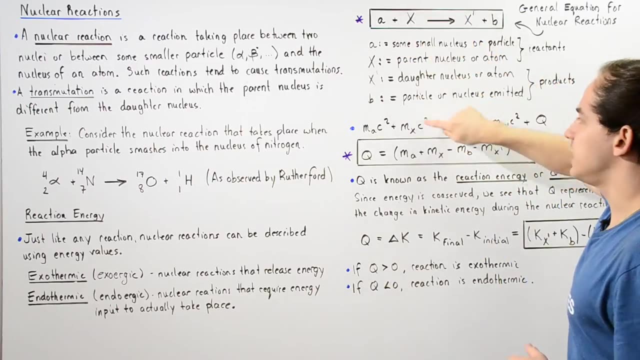 holds in any nuclear reaction, and that means we can write the following equation: So basically, on the reactant side we have the sum of our rest mass energies of our particle A as well as our parent nucleus X. Now this is equal to the rest mass energies of these two quantities. 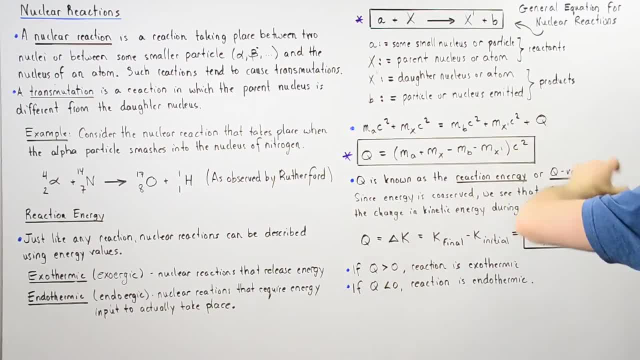 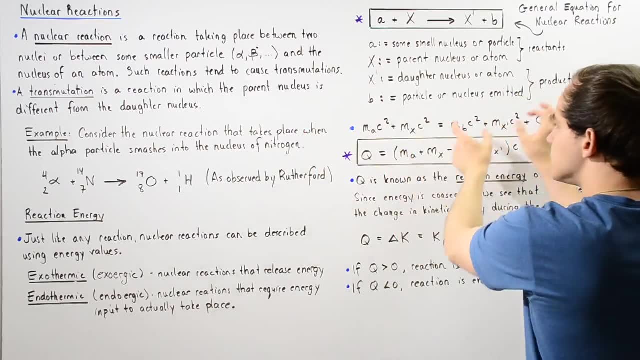 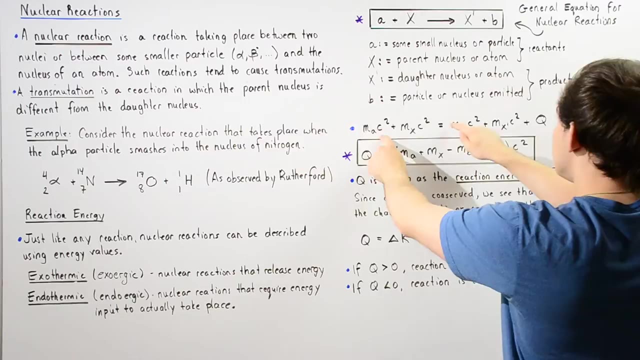 given here plus Q. Now Q can be solved and we get the following results: So this is the, So Q is equal to. we take these and bring these to the reactant side and we get the following result: Now, because we have the C squared term that appear in every one of these quantities, we can take that out and we get the following result. 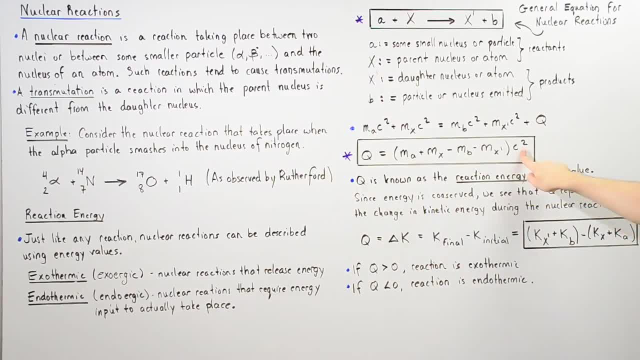 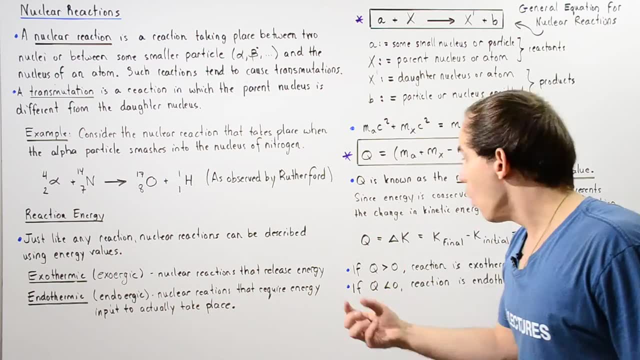 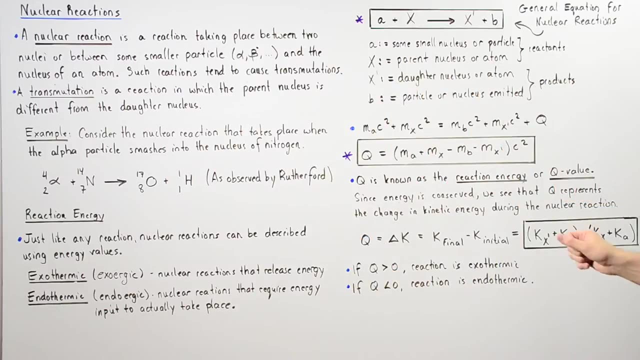 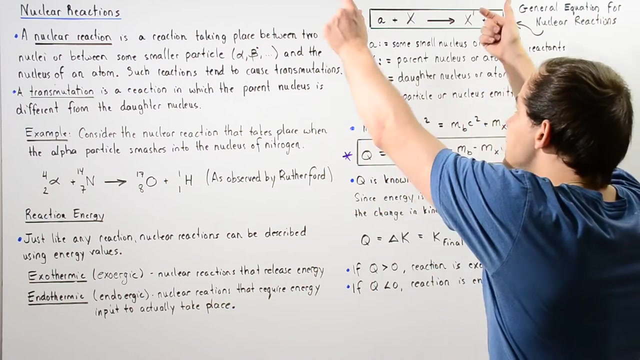 So we take the difference of the masses and multiply that by C squared and that gives us our Q value. Now Q is simply the Q value or the reaction energy of our nuclear reaction. And by the conservation of energy we see that Q simply represents the change in kinetic energy that takes place when our nuclear reaction takes place. 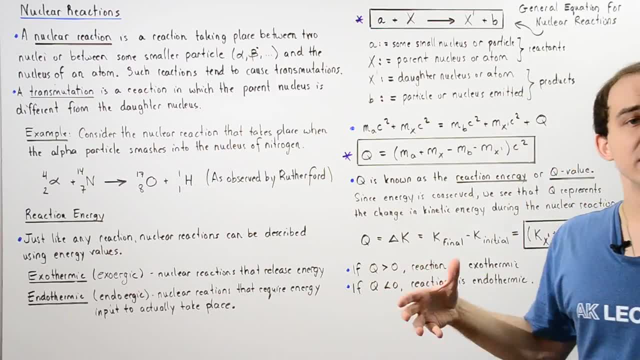 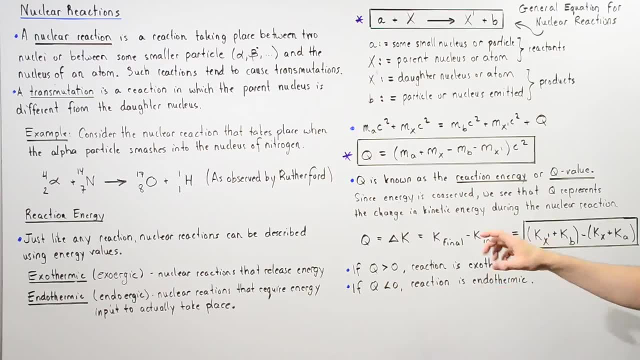 So Q is simply given by the change in kinetic energy. It's the kinetic energy of the final product minus Q, The kinetic energy of the initial reactants. So we have the kinetic energy of X, prime and B. We take the sum and subtract the sum of the kinetic energies of the reactants. 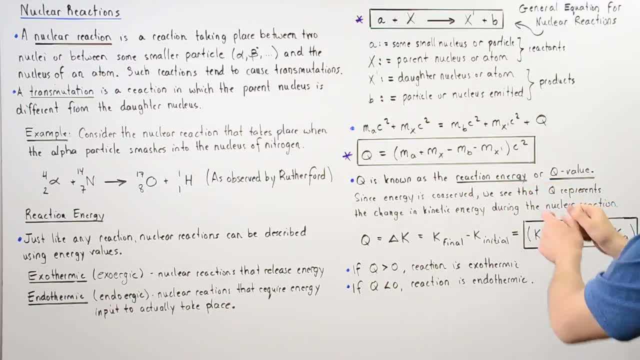 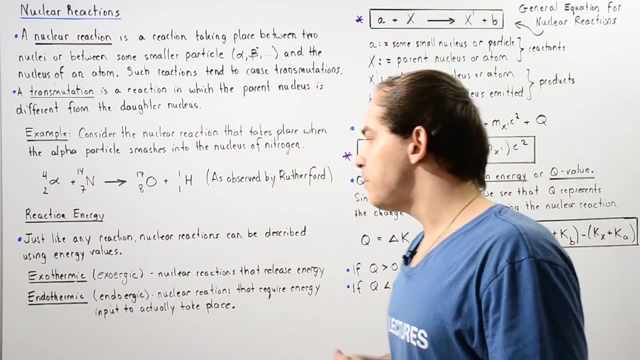 So this gives us the reaction energy. So we can either use this reaction or we can either use this equation or this equation to calculate what the reaction energy is. Now, whenever Q is a positive value, That basically means our nuclear reaction is an exothermic or an exoergic reaction. 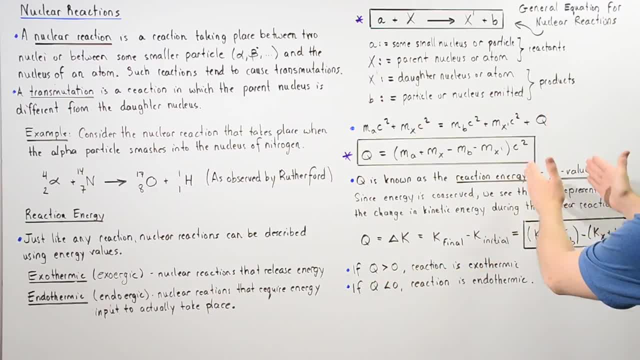 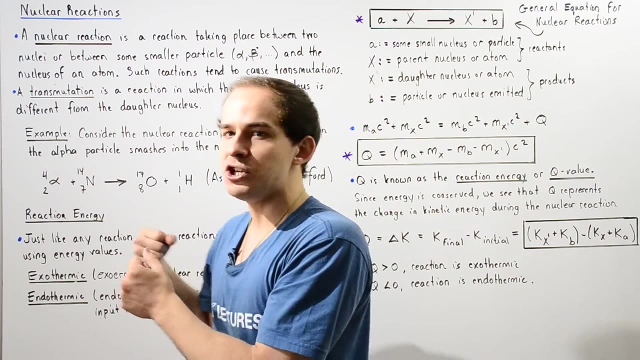 And if Q is positive, that means that the final kinetic energy of our two products is greater than the initial kinetic energy of our two reactants. So that means when the reaction takes place, energy is released and that energy is gained by the kinetic energy of our two products. 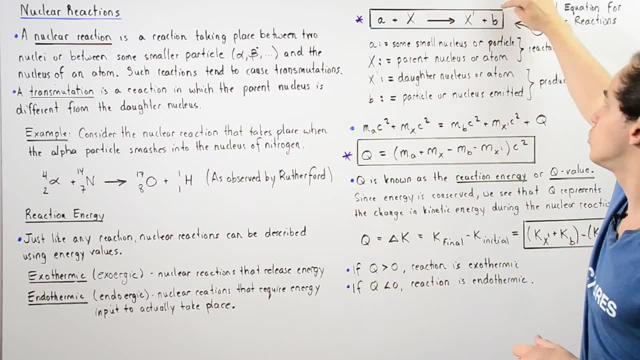 And that energy is released and that energy is gained by the kinetic energy of our two particles of our nucleus: the daughter nucleus and particle B. Now, on the other hand, if Q is negative, that basically means that this quantity, the sum of the kinetic energy of the reactants, is greater than the sum of the kinetic energy of our two products.